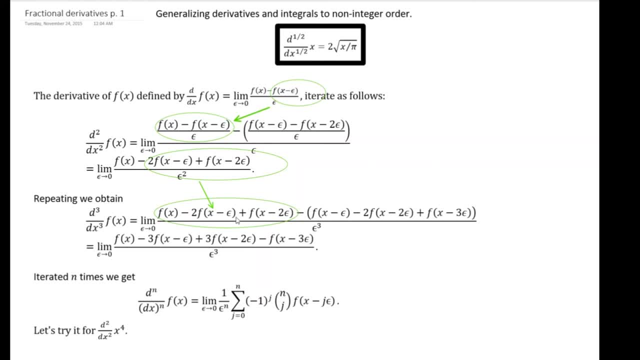 versus: here x x minus epsilon, here x minus 2 epsilon, here x minus 3 epsilon. and we simplify the algebra, we get this And, if you're beginning to notice, the binomial series is beginning to happen. Here's 1, 3, 3, 1.. 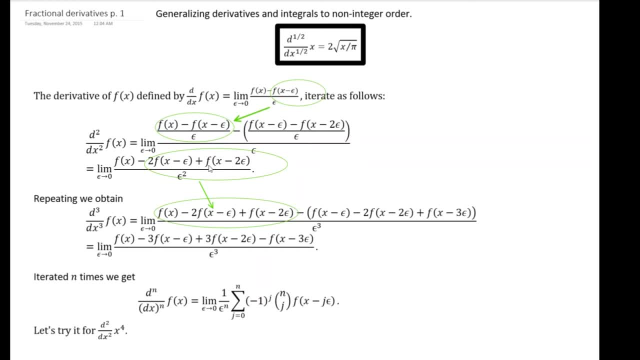 And this is 1, 2, 1. Pascal's triangle right. So if we iterate this differentiation process n times, we can demonstrate- We can demonstrate to ourselves inductively- that what we're going to get is epsilon here. 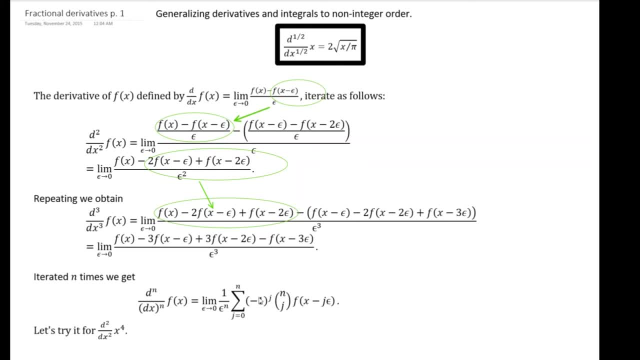 1 over epsilon to the nth, the sum of the alternating sign minus 1 to the jth, power of the binomial coefficient times f of x minus j epsilon, where j is counting from 0 to n. This is counting integers And the best way to prove or at least feel comfortable. 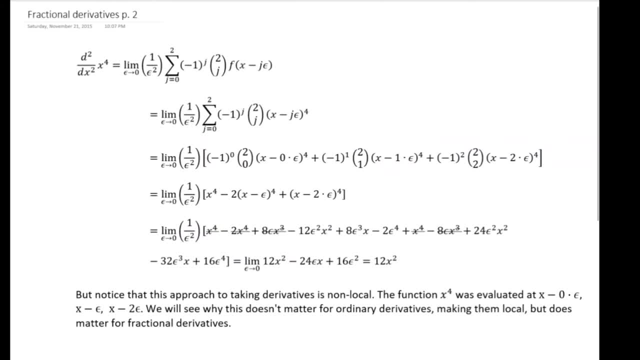 that this is true is to consider, say, the derivative of x, x to the fourth. Let's take the second derivative using this formula that we have right here. Fine, So we're going to have 1 over epsilon squared, We're going to have the sum going from 0 to 2,. 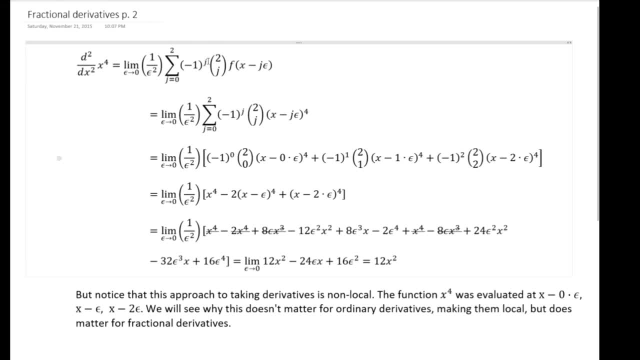 negative 1 to the jth binomial coefficient, 2 over j, where j is going to go 0 and 1 and 2, and f of x minus j epsilon. There it is substituted in with f of x minus j, epsilon being. 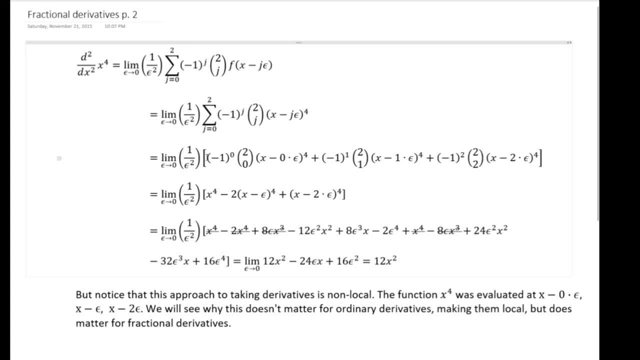 x minus j. epsilon parentheses to the fourth power. Let's go ahead and expand out the series. here We have one, the first term, the second term and the third term, And when I simplify things, I'm going to get x to the fourth power. 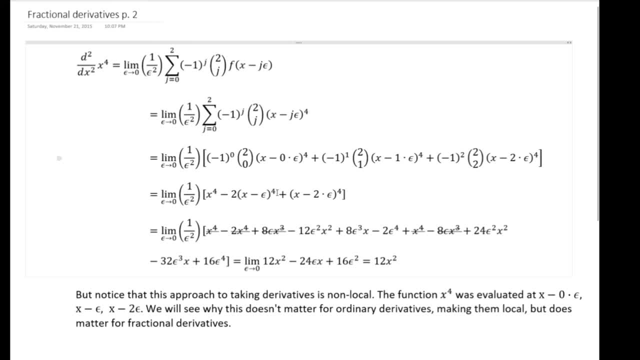 minus 2 times x minus epsilon to the fourth power, plus x minus 2 epsilon to the fourth power, And I clean up all my algebra. And what remains after all this cleaning up is 12x squared minus 24 epsilon x plus 16 epsilon squared. 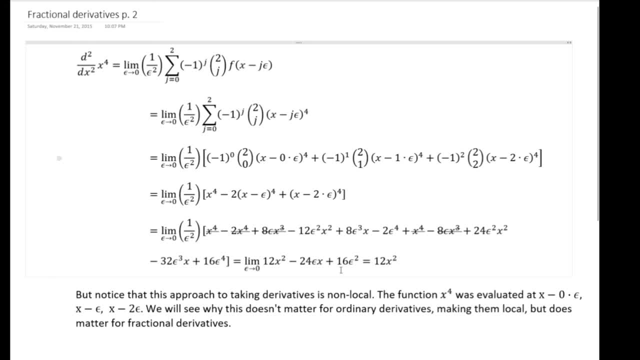 And, of course, when I take the limit- as epsilon tends to 0, I get 12x squared And we know that if we take the first derivative of this, we would see 4x cubed and the second derivative would give us 12x squared. 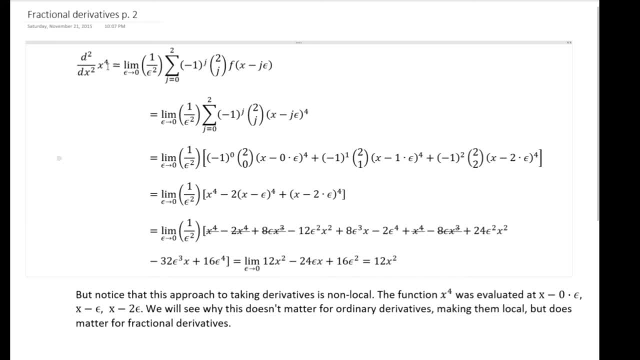 It's following exactly what we would get with the regular calculus. Except here, instead of taking the derivative locally, we might take the derivative and evaluate it at some point. x naught. We're actually creeping along the function. We have x, We're at x and then we're sliding over. 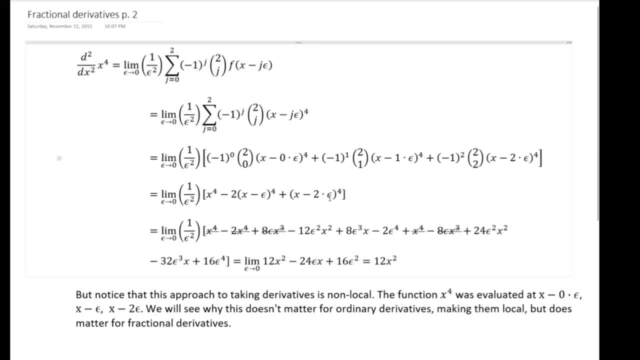 shifting by minus epsilon and shifting by minus 2 epsilon and up here all the way up to the jth value of epsilon. So this is not a local version of the differential calculus And we'll see how that affects things in a few minutes. 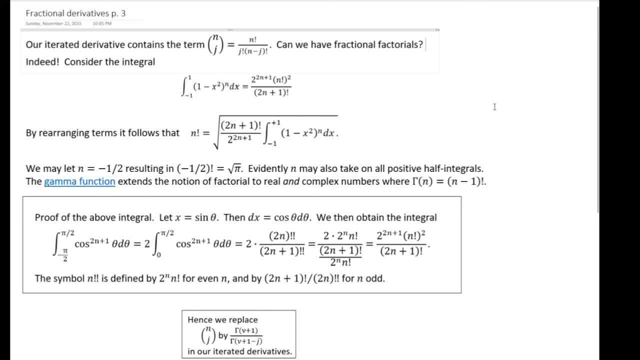 Here comes the connection to how we can take derivatives with a fractional, fractional derivatives, that is, We have this symbol, This is the binomial coefficient that we all know: n over j here really is defined as n factorial over j factorial, n minus j factorial. 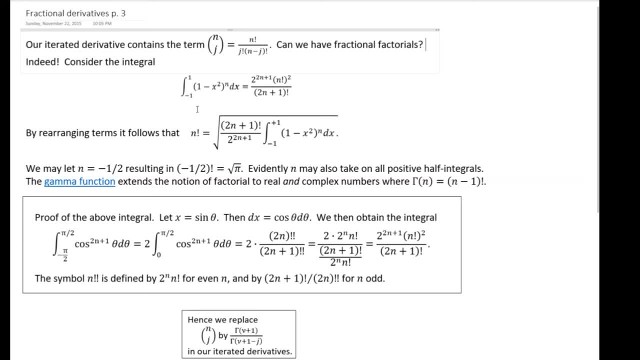 This is an integral which I will prove below, in the box below that, the integral from negative 1 to 1, of 1 minus x squared, that quantity raised to the nth power, dx, is equal to this. For now let me just solve algebraically for n: factorial. 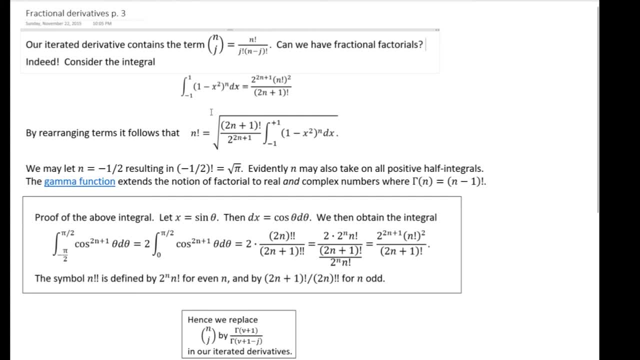 I put this over here and this under here and I take the square root and I have a formula of n factorial that's based on an integral from negative 1 to 1 of 1 minus x squared to the nth power. 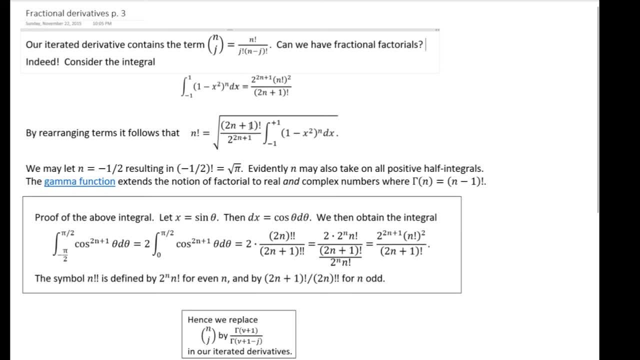 the quantity to the nth power, and with these factorial and powers of n here. And in fact, if you say let n equal to negative 1 half and do the integral, you would get square root of pi. So there we have a fractional factorial. 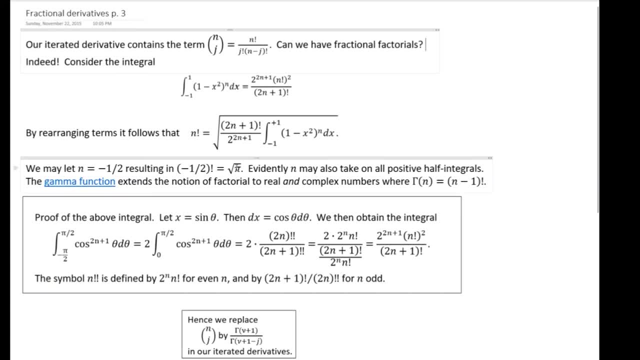 and related to the square root of pi. So let's go ahead and prove that integral. We let x equal to sine theta and therefore dx is equal to cosine theta, d, theta, And so naturally this becomes 1 minus cosine squared can become sine squared to the nth power. 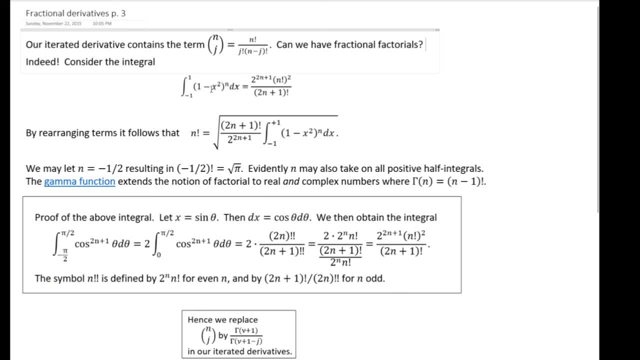 and that's 1 minus sine squared, squared is 1, sorry, that meant cosine. 1 minus sine squared is squared is 1, is cosine squared. And then we have the cosine theta d theta. so it becomes cosine to the 2nth plus 1 theta d theta. 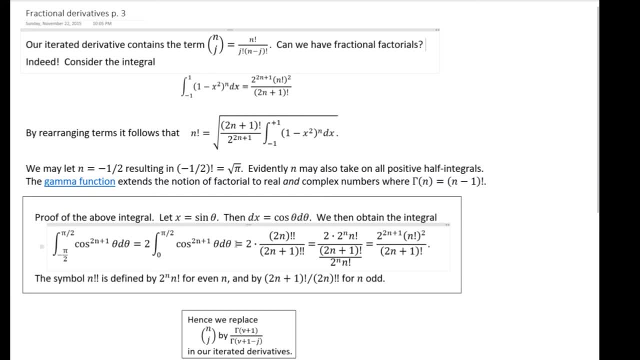 And you can look this up as a table integral, or do it by induction, You can do it to, You can just plug in n and iterate, and iterate and iterate and convince yourself that this is the formula that will happen, or you can do it by induction. 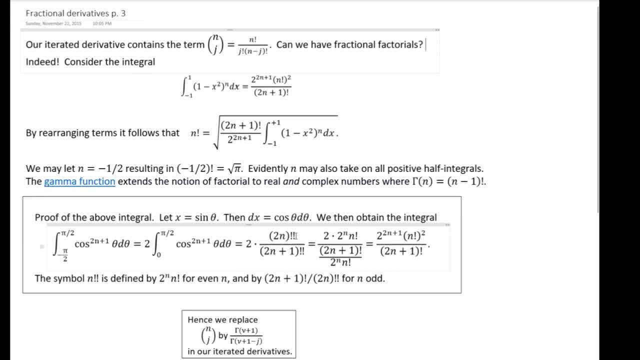 And you're gonna get 2n and you're gonna get the quantity to the double factorial, And the double factorial is defined by: you replace it by 2 to the nth n factorial For if n is even, and you replace it by 2 to the n plus 1 factorial. 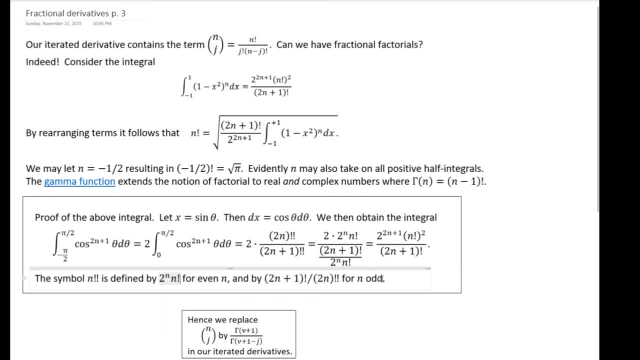 over 2 to the n factorial, factorial for if. n is odd, And so once again we have exactly what we had up here. If I solve for n, I get 2n plus 1 over here on top, and I get 2n plus 1 over here on top. 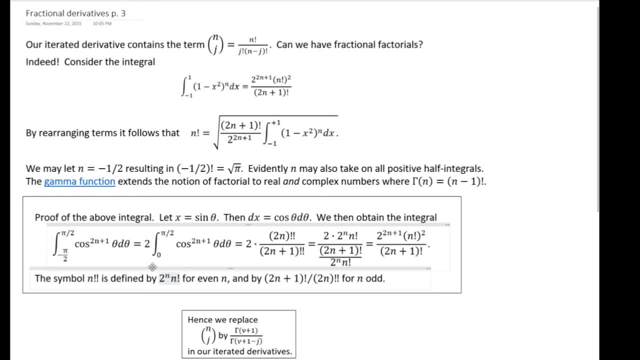 And I get 2 to the 2 nth plus 1 on the bottom and I take the square root and this integral is really the same thing as that integral. So I now have the right To replace the symbol where n and J the binomial coefficient where n and J have been integers all our life. 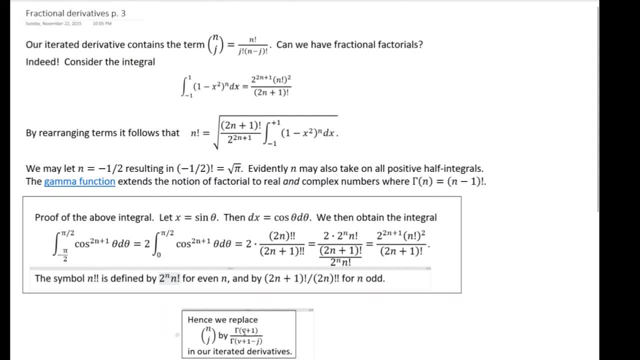 By the gamma function and you should look that up. the gamma function of n is n minus 1 factorial. So I'm making that connection Right here And you should look up the gamma function. I'm using the gamma function to replace the binomial coefficient, So instead of having and 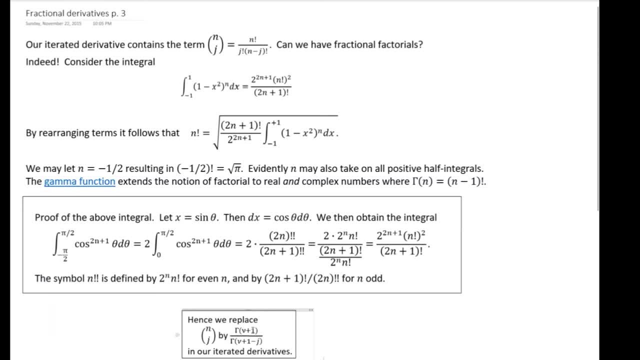 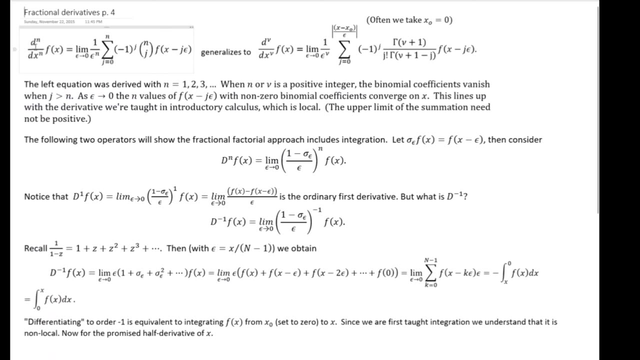 I've now have gamma to the nu plus gamma of nu plus 1 and J is gamma as nu plus 1 minus J. So this is going to allow me To take my iterated derivatives, where I was doing first through this second derivative to get to this binomial. 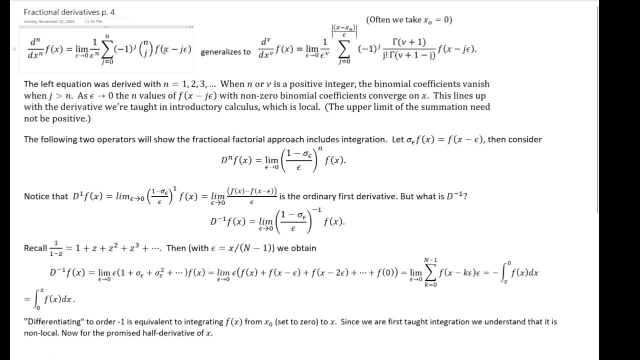 expansion, these by no coefficients here, and An expansion of the derivative in terms of f of X sliding along 0 epsilon, 1 epsilon to epsilon, Which we proved gives us the derivative of X to the fourth power. The second derivative gives us it, gives it to it us, correctly. 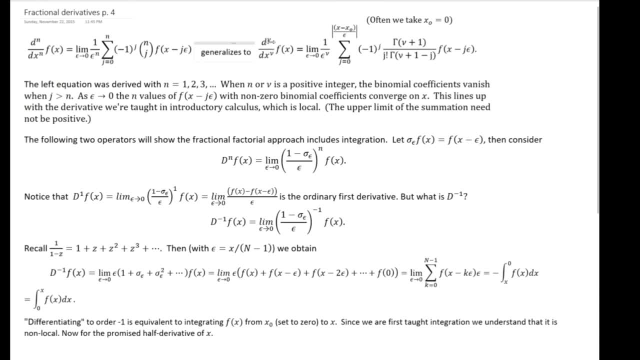 Now it generalizes to the NU state, derivative D to the dean youth. the extra news f of x. I still have the limit, but it's now 1 over epsilon to the newth. And now the sum. you see what's changed here. 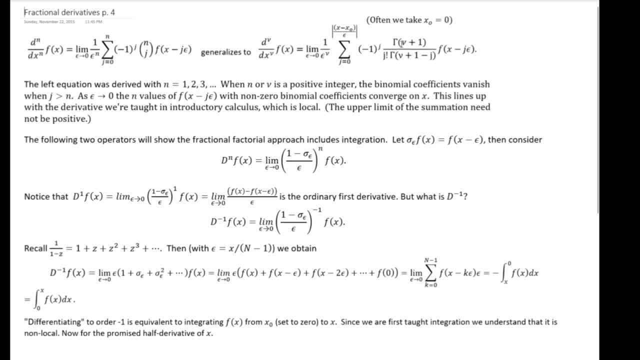 I replaced this symbol, the binomial coefficient, with the gamma of nu plus 1 over gamma of nu plus 1 minus j. Everything this is the same. The jth factorial is here and the alternating sign is here, And now I'm about to move into away from. n equals 1,, 2, 3.. 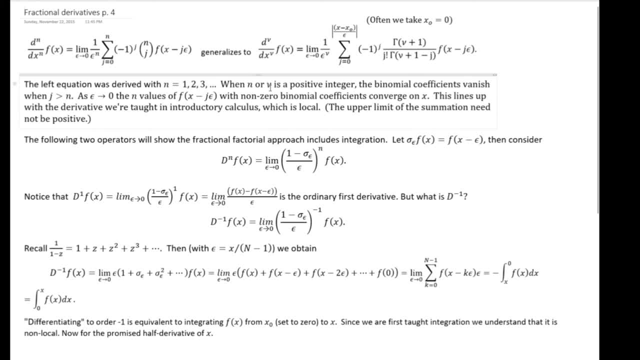 1,, 2, fractional. So when n or nu is a positive integer, the binomial coefficients vanish. when n exceeds j, Sorry, when j exceeds n, that makes sense. When this is greater than that. that's it. And as epsilon tends to zero the values of f of x minus j, epsilon. 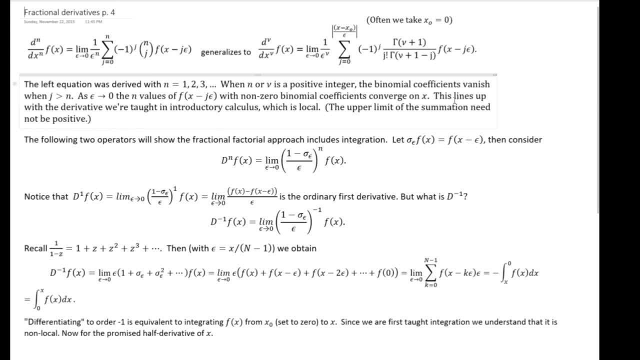 with non-zero binomial coefficients converge on x. This just lines up with the local definition of derivatives And, by the way, I took the absolute value here. It need not be, It need not be positive. So let's pay attention to this really carefully. 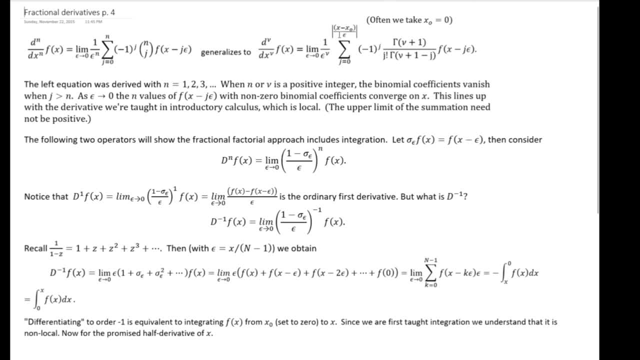 In the simplest form of integration, we partition a function into equal-sized rectangles of equal width and variable height when we're doing the Riemann sum approximation. So here I have the interval from x to x0 divided by epsilon. Okay, so I'm going to define a new operator. 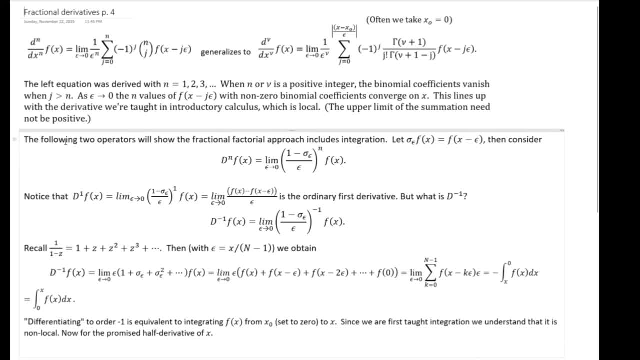 I'm going to show you that positive fraction. And if the fractions correspond to the differential calculus, the fractional differential calculus, and if the fractions become whole numbers, then we have just the calculus that we were taught. But if we have negative powers, we actually have the integral calculus. 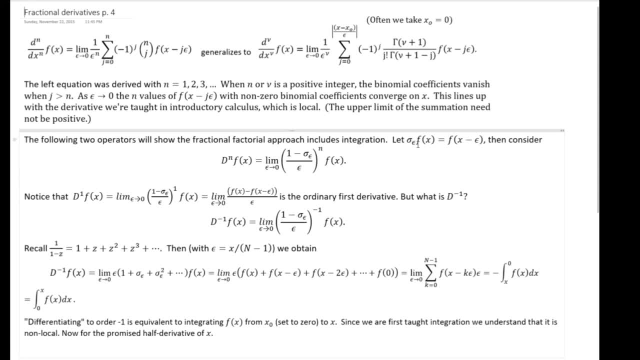 So this operator, here sigma sub epsilon, operates on f of x. by changing it to f of x minus epsilon, It's a shift operator. Consider the nth, Consider d to the nth. being operating by this operator n times. And we define it as the limit, as epsilon tends to 0, 1 minus epsilon, sigma sub epsilon over epsilon to the nth power f of x. 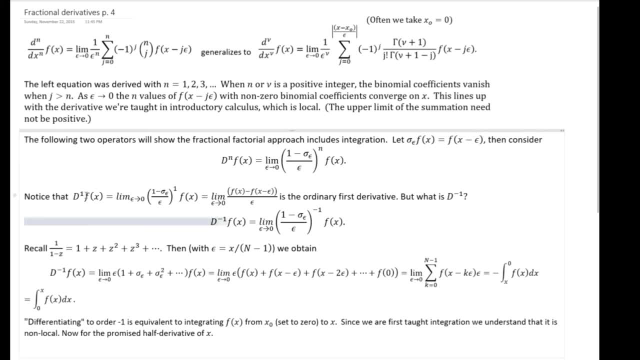 Let's test out this operator. Let's do the simplest case, Let's do the first. So I'm going to have the limit, as epsilon tends to 0, 1 minus sigma, sub epsilon, over epsilon, to the first power times f of x. 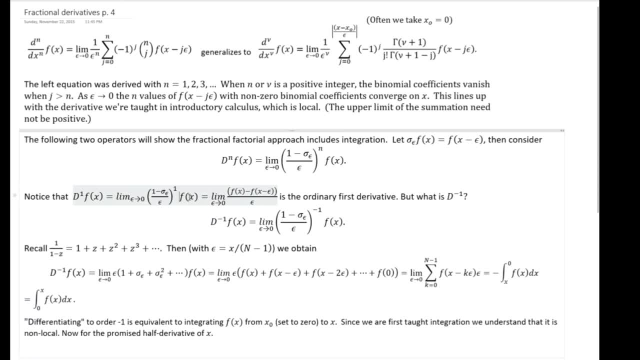 And I just plug in what the operator tells me. It says: oh, f of x distributed to the 1 gives me f of x. f of x being hit by that operator gives me f of x minus epsilon. I divide by epsilon. 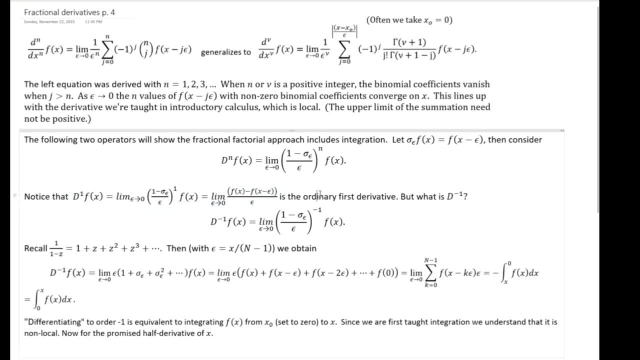 As epsilon tends to 0,, I get back my ordinary first derivative And please do this for the second and third and fourth derivatives to convince yourself. this is just a fancy way to write this formula right up here. It's a fancy way to write up that formula with this operator. 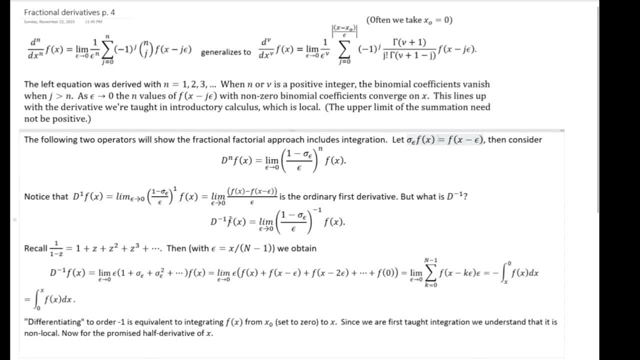 Now consider the operator to the negative 1 operating on the function f of x As the limit, as epsilon tends to 0, 1 minus sigma sub epsilon over epsilon. to the negative 1 f of x. Well, recall, so this is to the negative 1.. 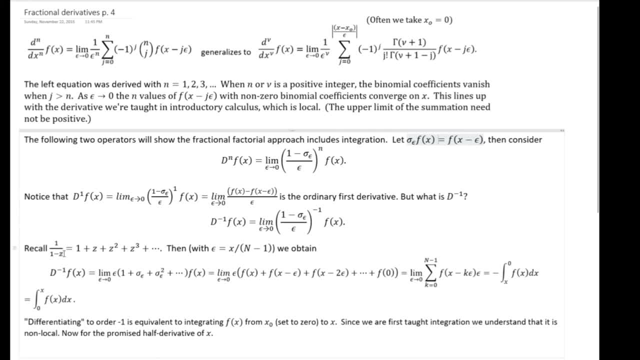 So this is really on the bottom right And in general, if I have 1 or 1 minus z, this is the expansion that I would get: 1 plus z squared plus z cubed. dot, dot, dot dot. 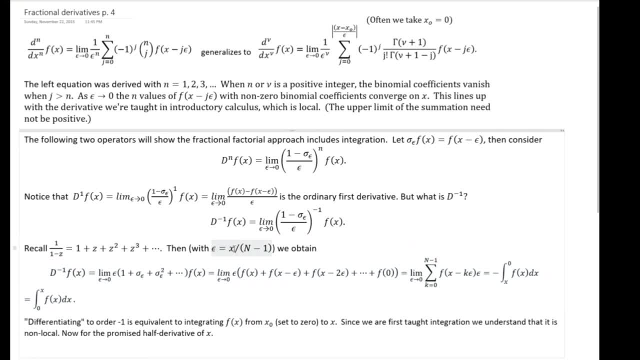 And then here's what I was talking about: If I have 1 over epsilon, consider it to be some width Divided by n minus 1, where n is the total number of intervals, Then this is a fixed increment. So now look at this. 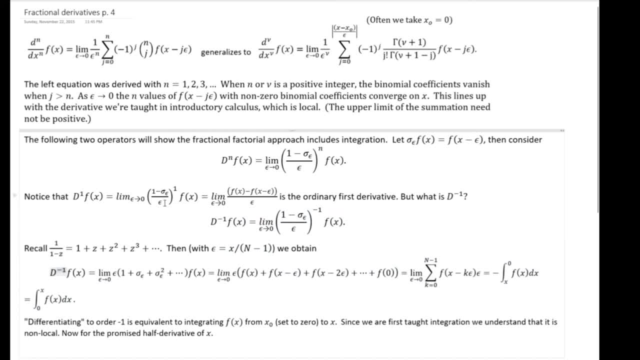 D to the minus 1 f of x is equal to epsilon, because the epsilon is going to go to the top. This is to the negative 1 power. so it's up top. This is to the bottom where I'm going to have my expansion here. 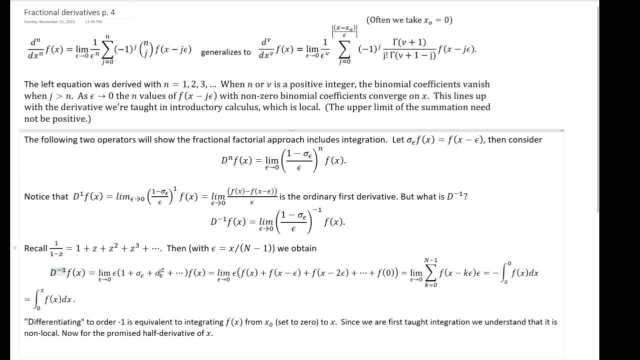 1 plus sigma sub epsilon, plus sigma squared sub epsilon, plus dot, dot, dot f of x, And if I operate that f of x times that, I get f of x And then that gets me 1 shift. There it is. 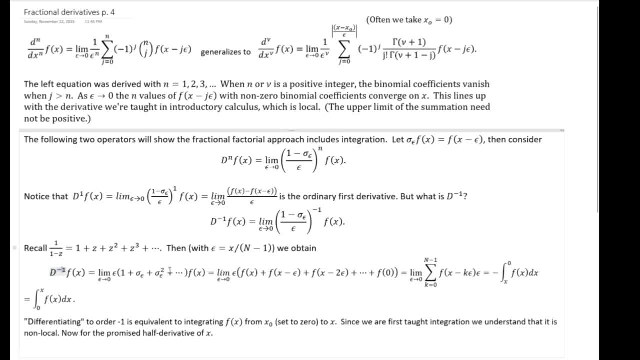 That gets me 2 shifts And I keep marching all the way until I finish at f of 0. Because I start at x and I'm moving to the left, Keep moving to the left, 2 epsilons And eventually I get to 0. in this case, 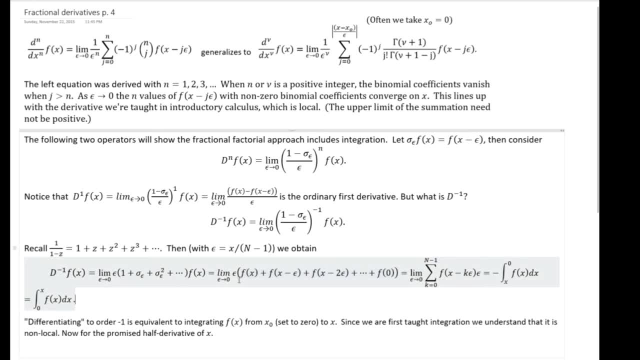 And so I look at this. I get the limit, as epsilon tends to 0, of f of x Minus k epsilon times epsilon, Where epsilon is the width. Think of that as your delta x And f of x is moving along. 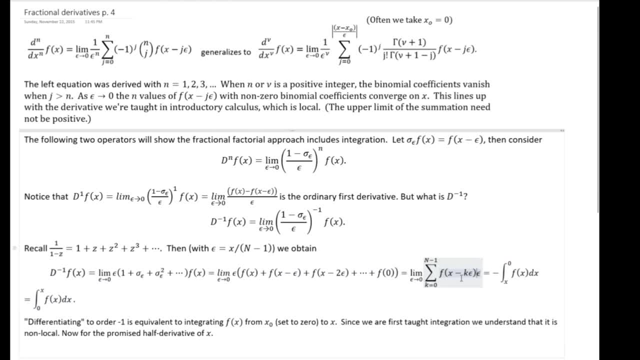 You're building rectangles of height f of x minus k, epsilon. Is that not this integral? And there we go, And if I just replace the minus sign over here, I get the integral from 0 to x of f, of x, dx. So there you have it. 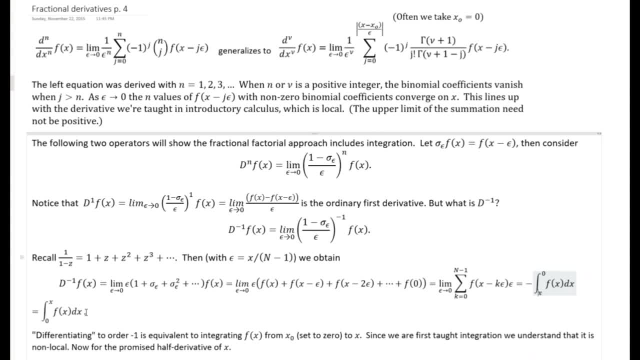 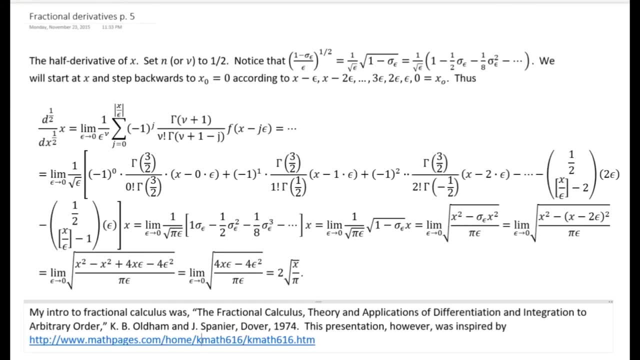 If you differentiate to the negative 1, if, that is, you take the negative 1 derivative of a function, you're actually taking its integral, its first integral. So now we get to what I promised you: I'm going to take the 1 half derivative of x. 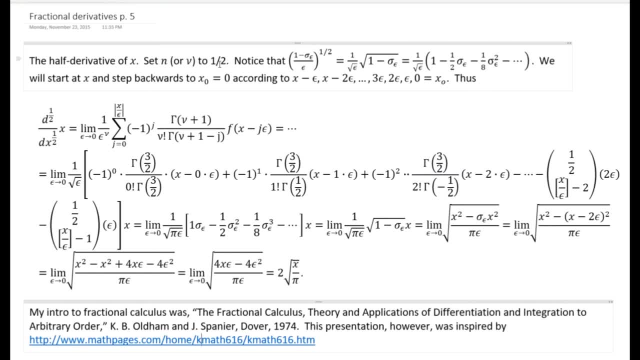 So I'm going to set n, or really nu, to the 1 half, to equal to 1 half, And I'm going to look at this operator here: 1 minus sigma sub epsilon over epsilon to the 1 half. Well, that's the same as 1 over the square root of epsilon, isn't it? 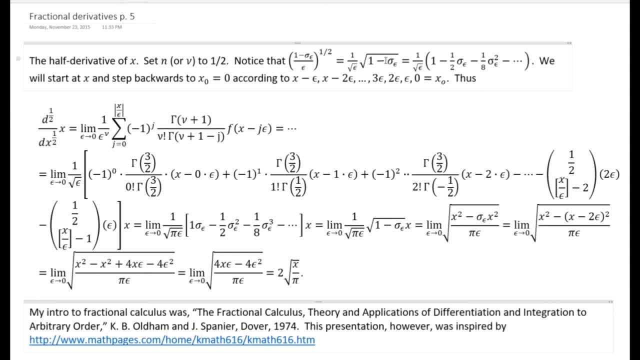 And square root of 1 minus epsilon, And that has an expansion of 1 minus 1 half epsilon minus 1. eighth dot, dot, dot, dot dot. We're going to start at x and we're going to step backwards to the initial point. 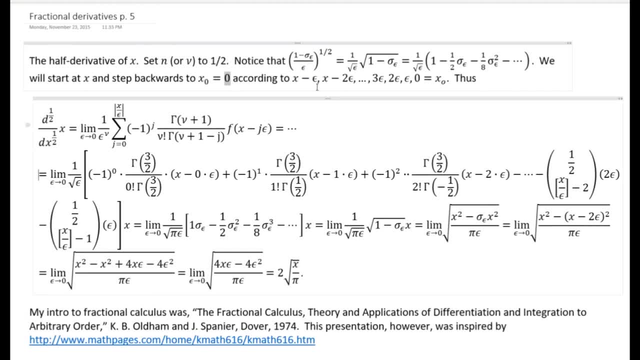 which, let's say, call it 0.. And so our steps are going to be: we're going to go to the left by an epsilon, by 2 epsilons, by 3 epsilons, until we eventually get 3 epsilons away from 0, 2 epsilons away from 0, 1 epsilon away from 0. 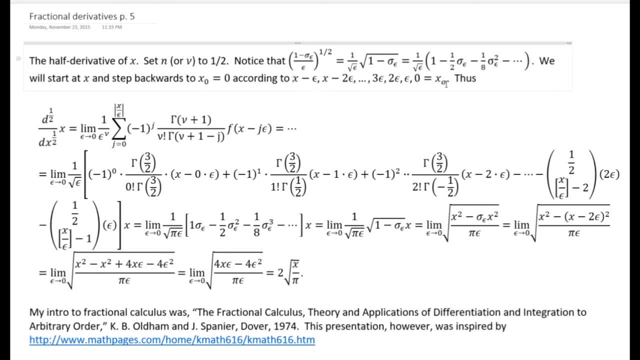 We are 0, at 0,, our initial point that we chose. So here we go. The 1 half derivative of x is the limit, as epsilon tends to 0, of 1 over epsilon to the nu And our, and how many integrals, how many intervals we're going. 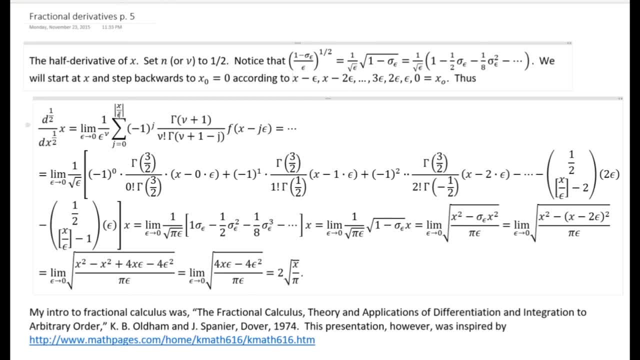 to do is x divided by this, fixed with epsilon, And we're going to sum from starting from 0.. Total weight of that: here's our alternating minus 1 to the jth power. Here's our gamma functions and here's f of x. 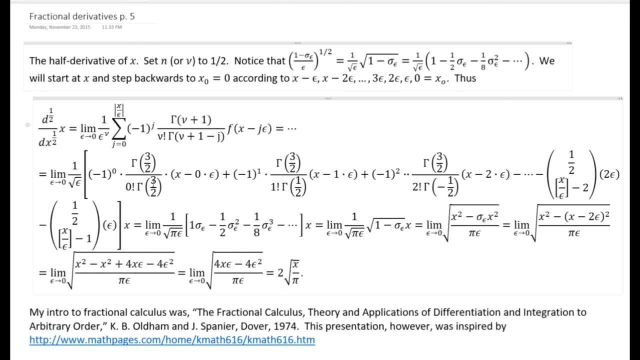 So let's do it At 0,. we have gamma to the 3 halves, 0 factorial gamma, 3 halves. There's our, there's f of x minus 1 to the first power. gamma 3 half, gamma 1 half.